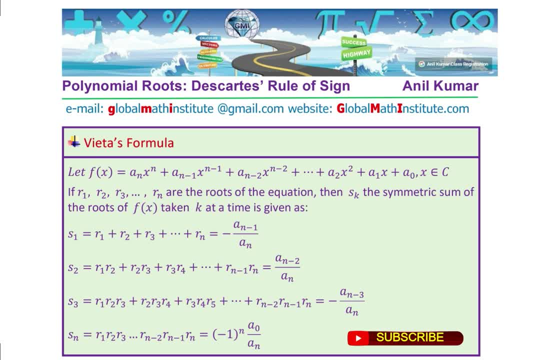 of the roots of functions taken, K at a time is given as this. So that means that if all the roots are added up, there is the ratio of leading An minus 1 over An with a negative sign Right. So sum of all the roots. 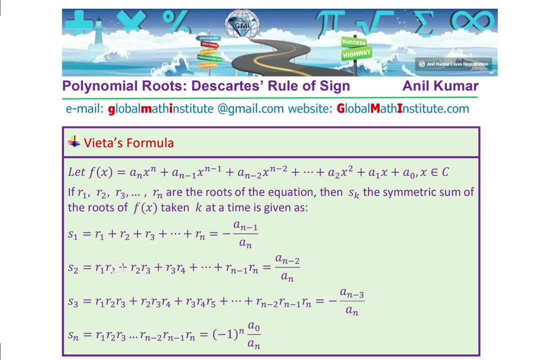 The sum of all the roots And the sum of product of two roots taken at a time will be a n minus 2 divided by a n, and so on. The signs alternate. At the end, what you get is the product of all the roots, which is a 0, the constant divided by the leading coefficient, a n. 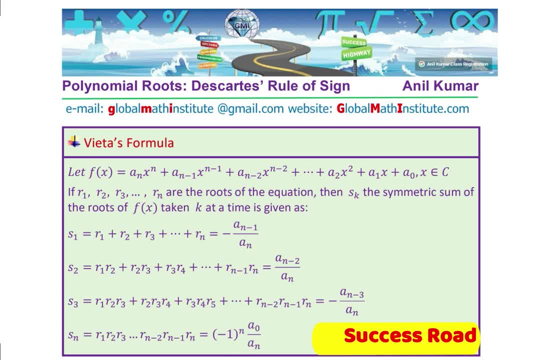 It will be negative 1 to the power of n, That is, if the polynomial of degree e1,, then this is positive, otherwise negative. Correct, So we can actually get the sum using the symmetric sums of the roots. So with that in mind, I think now clearly you can answer these questions. 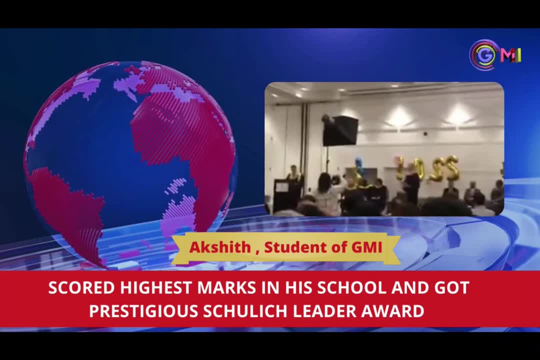 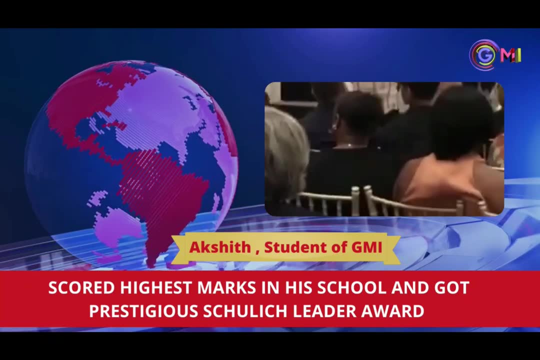 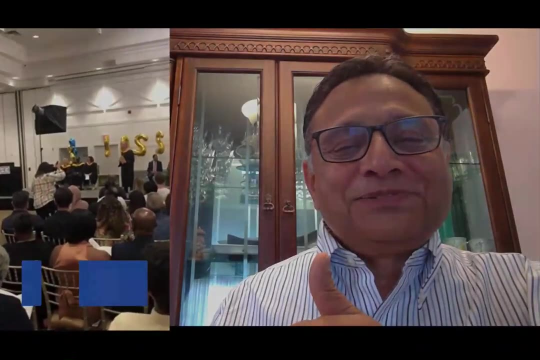 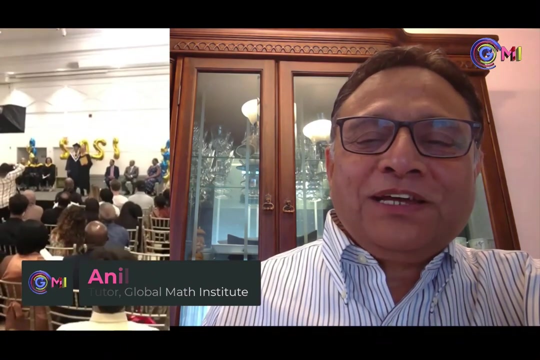 After attending university. the winner of this year's Certificate of Achievement, Schulich Leader Award, is Akshi Khenjilani. Great, Our student Akshit gets highest marks and the most prestigious Schulich Leader Award. You can be there. 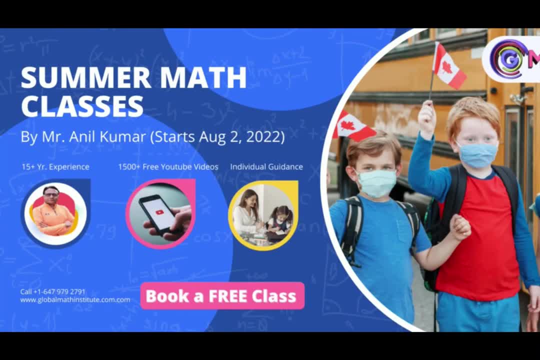 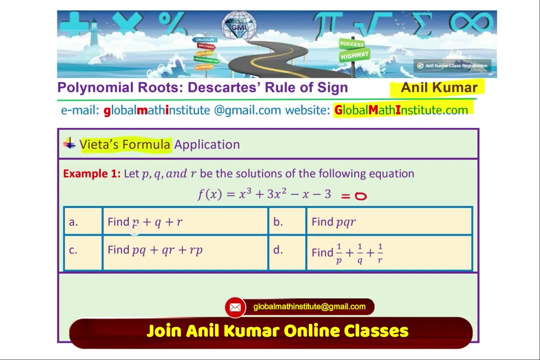 Join our classes and excel. Let's do them one by one. Part: A Sum of the roots. right Now here. in this case, we know that a3 is 1.. Then a2 is equal to 3.. a1 is minus 1.. 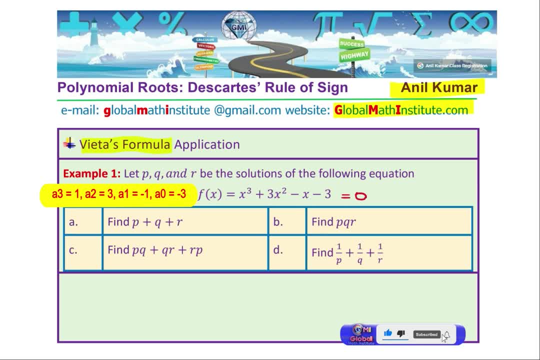 And the constant, which is a0, is minus 3, right. So what are the sum of the roots? Sum of the roots is 3, right, 3 divided by 1.. So sum of the roots is equal to negative sign because it is cubic right. 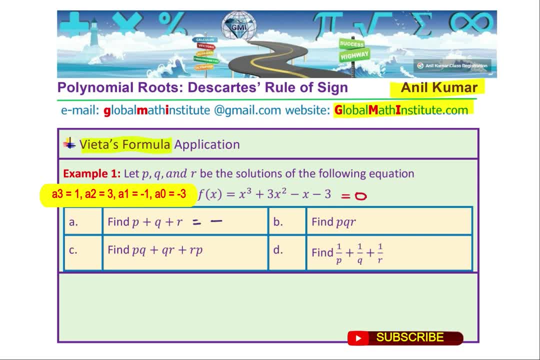 So starting, everything is negative, So it is negative 3. The product of roots is a0, the constant and the sign will be: 1. Negative, positive, negative, right, Negative of this, So it is negative. of negative, 3, which is positive, 3.. 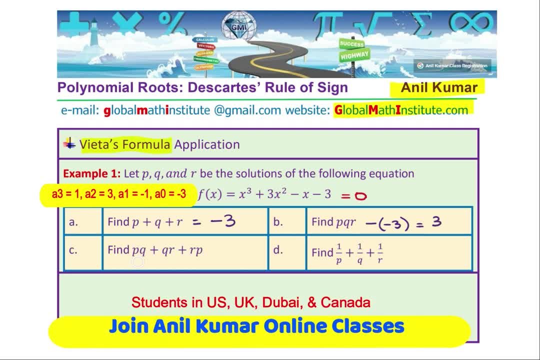 You see that The symmetric sum of product of two of these will be pq plus qr plus rp, will be the coefficient of x divided by a. So in this case it is going to be equal to minus 1,. right Now, how do you find 1 over p plus 1 over q plus 1 over r? 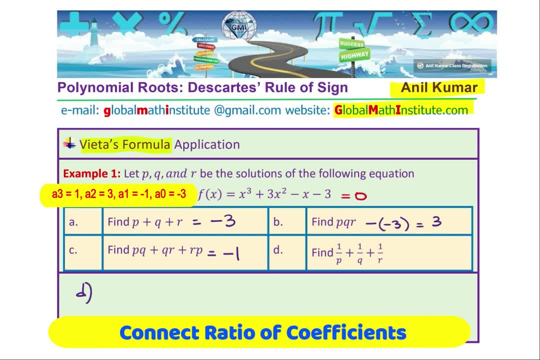 So for part D, let us find what is: 1 over p plus 1 over q plus 1 over r equals 2.. We can take the LCM, which is pqr, product of roots, and then we have qr plus pr plus pq, right? 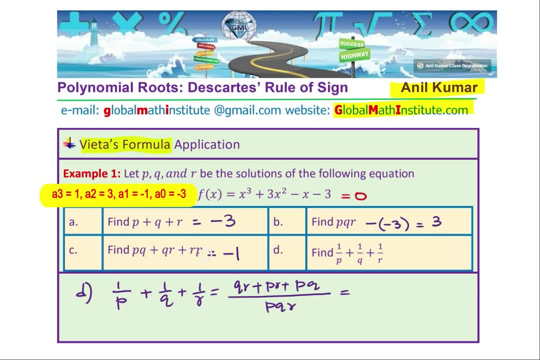 So that is the symmetric sum when two of them are multiplied, which is part C. So this is basically the ratio of minus 1, which we calculated in part C over b, which is 3.. So that is negative 1 over 3.. 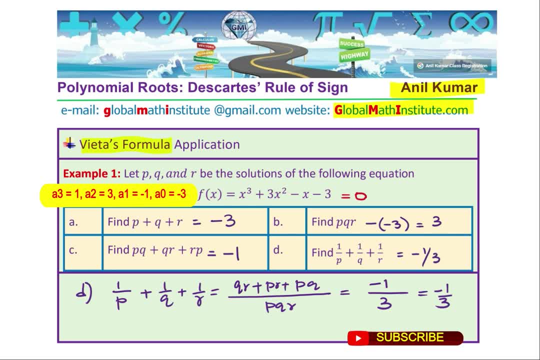 Is that clear to you? So, using Witter's formula, very easily we can actually find sum of roots, product of roots and different combinations, right? So that is how you could do it. Now you can actually verify the result by finding the real roots, right. 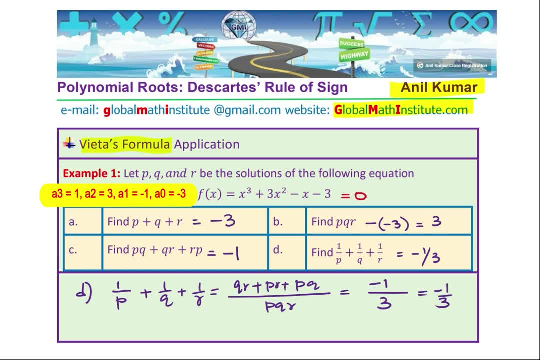 Write it in the factored form, correct, And then you will figure it out correct. So in general, you should also notice that a cubic equation like x cubed plus, let me write bx squared plus Cx plus d.